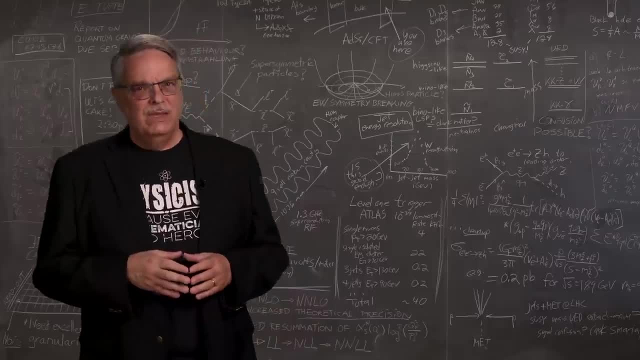 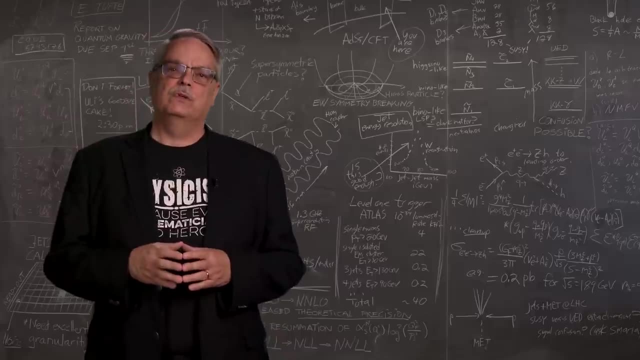 attempts to explain the subject in simple ways. Each idea has burrowed its way into the subconscious of people who are interested in science but aren't quantum experts. So what is quantum mechanics all about? really To understand that in any accurate detail? 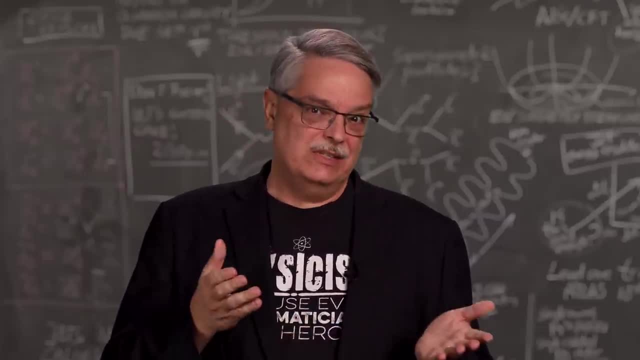 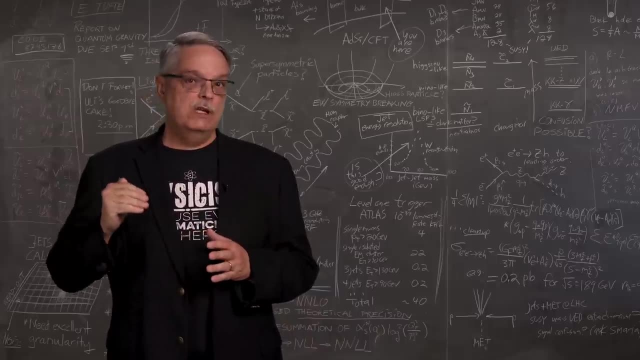 takes a ton of study, but I thought I'd try to boil it down to its essence in a single video. Perhaps we should start with a name. The word quantum implies a discrete quantity of something. For instance, the Sahara Desert can go on seemingly forever, But it's not. 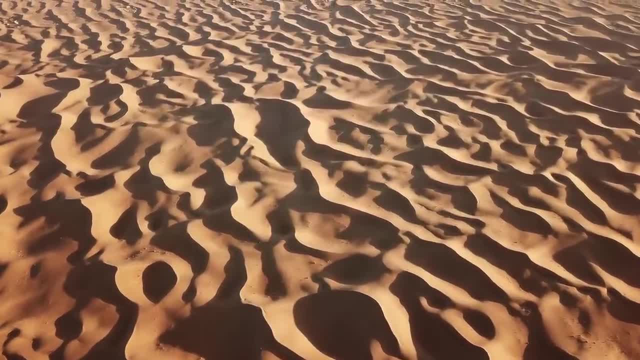 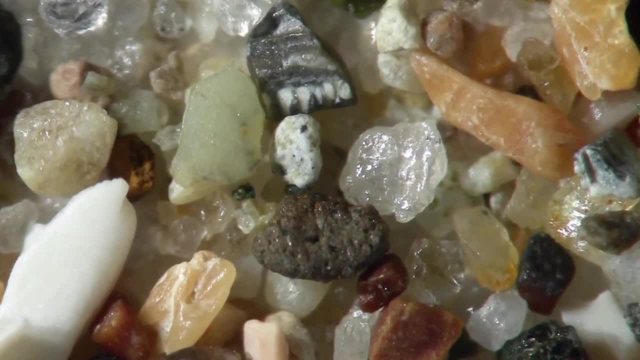 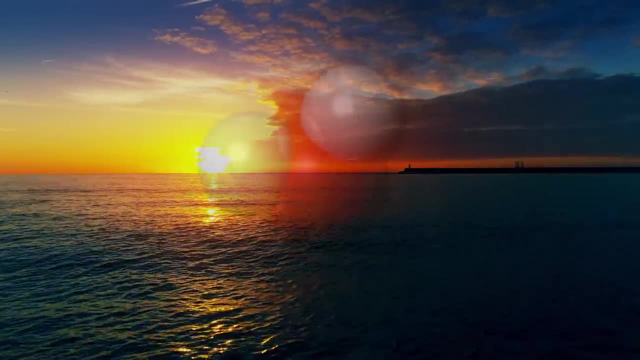 forever, with Dune following Dune. But as infinite as the sea of sand seems, it has a quantum side. The quantum of a desert is a single grain of sand. Alternatively, the ocean is majestic, liquid and in constant motion. There, the quantum is a single molecule. 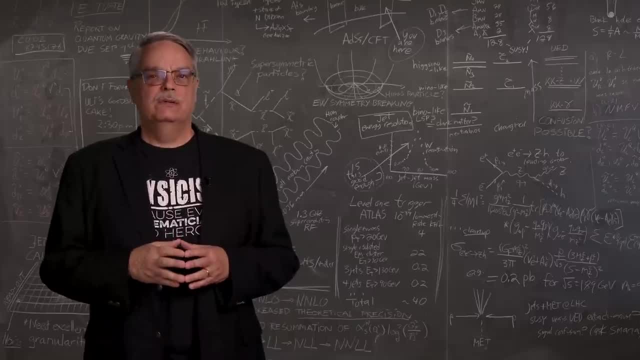 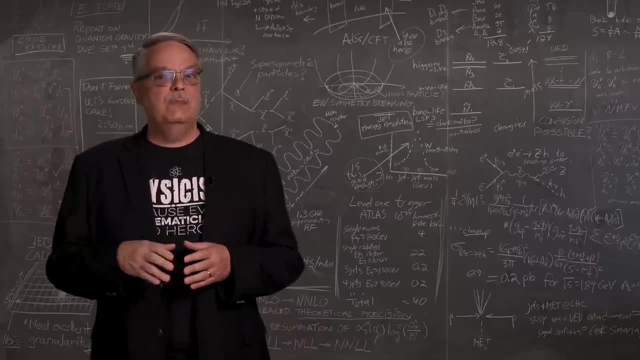 of water. So that's what quantum means. It means that we're talking about the smallest bit of something. The term mechanics is much easier. It just means the behavior of something. It means the behavior and motion of something. For instance, celestial mechanics means the motion. 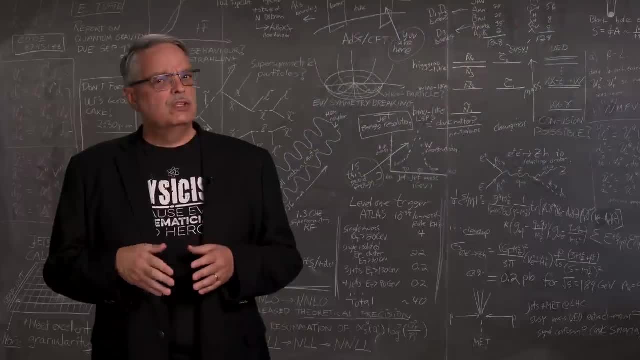 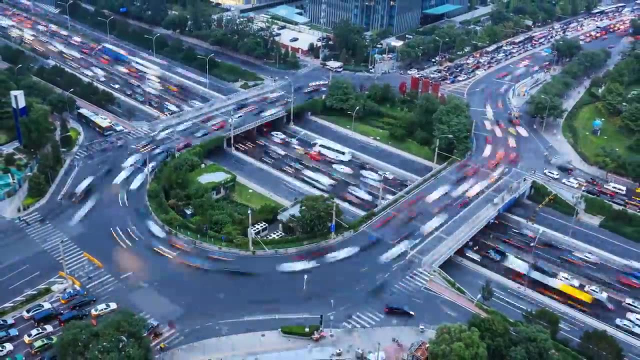 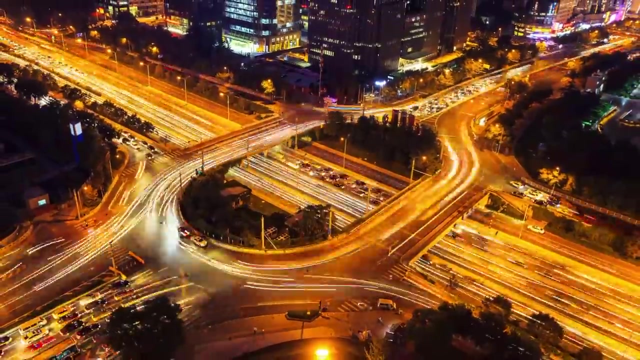 of the planets and other heavenly bodies. Thus, quantum mechanics is the motion and interaction of individual objects of a bigger collection. By that definition, the motion of an individual car on a freeway could be described as being governed by quantum mechanics, And of course that's not quite what we 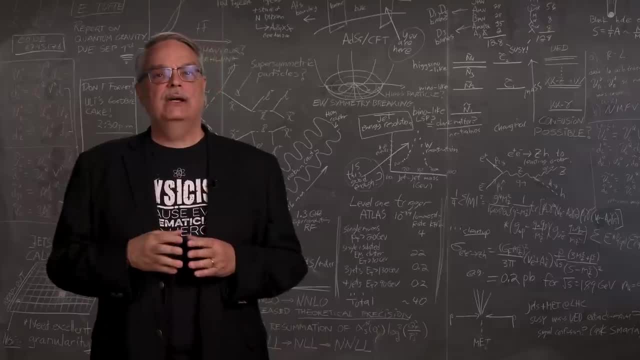 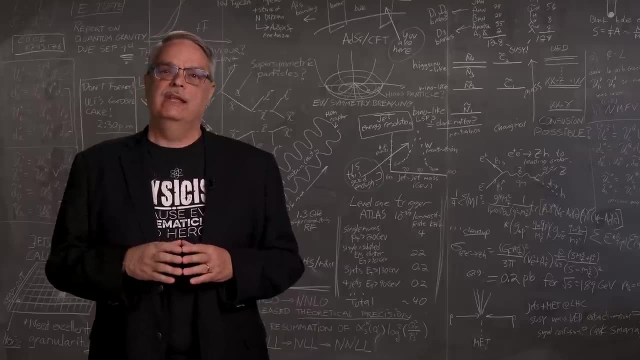 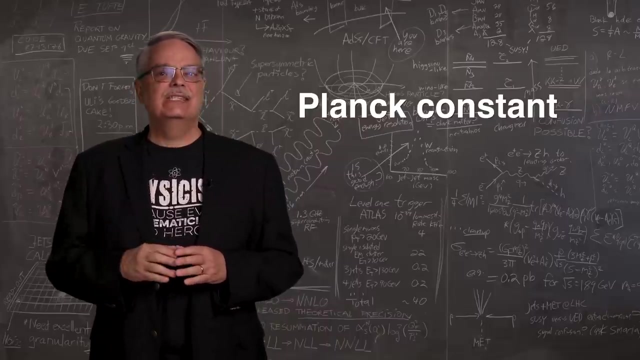 mean. In order to experience the counter-intuitive bits of quantum mechanics, we have to look at individual things that are very small, generally smaller than an atom. This is because quantum theory uses the Planck constant, which is a tiny number. It's this tininess that 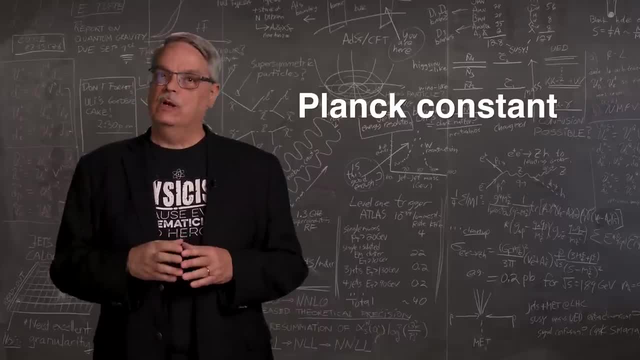 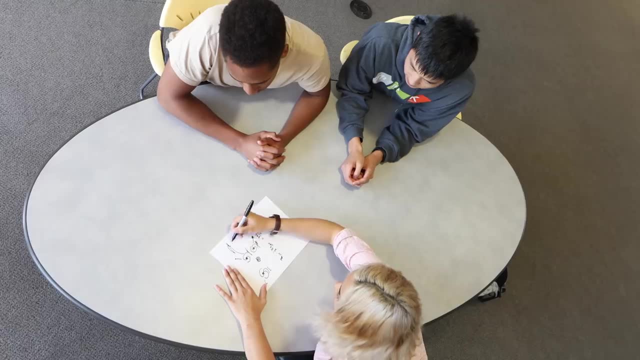 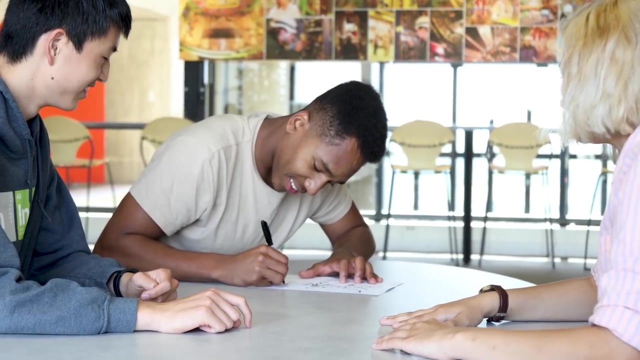 keeps the quantum weirdness constrained to the subatomic realm. When physicists first learn quantum mechanics as part of our training, we are studying the behavior of individual electrons surrounding atoms or individual photons of light. By and large, that is the realm of quantum mechanics. 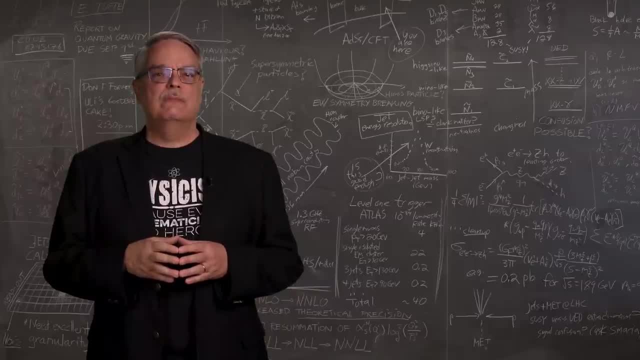 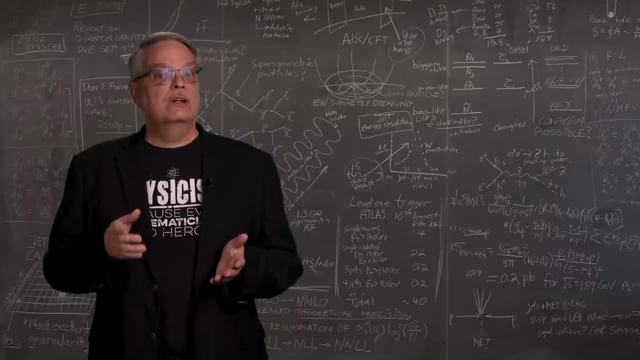 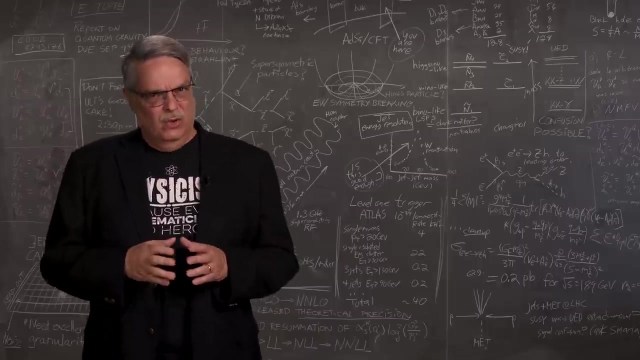 In a subsequent video, I'll talk about how the weirdnesses of quantum mechanics can manifest themselves on larger scales, But for now, let's talk about this world of the ultra-small, where we're talking about individual subatomic objects. OK, so now I need to introduce a key idea called the wave function At the subatomic level. 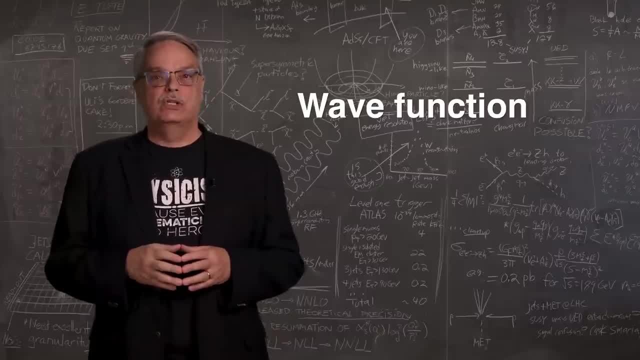 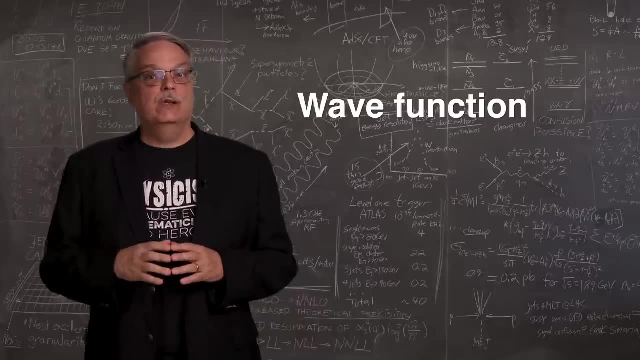 a wave function is a mathematical function that describes what is going on. It is called a wave function in part because for individual photons or electrons that aren't connected to an atom, the wave function looks like a familiar sine wave. There are other wave. 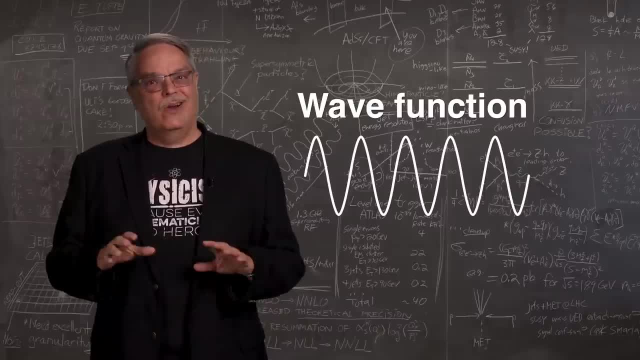 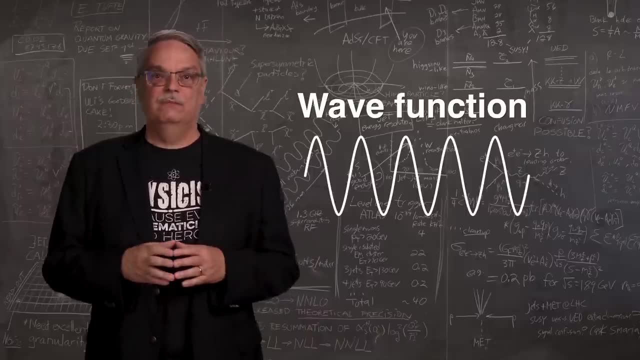 function shapes when electrons are near a nucleus, but the big ideas aren't dependent on the details of their shape. For simplicity, you can simply think of wave functions as sine waves. Now, that is the first curiosity. The sand grain or water molecule is a distinct and 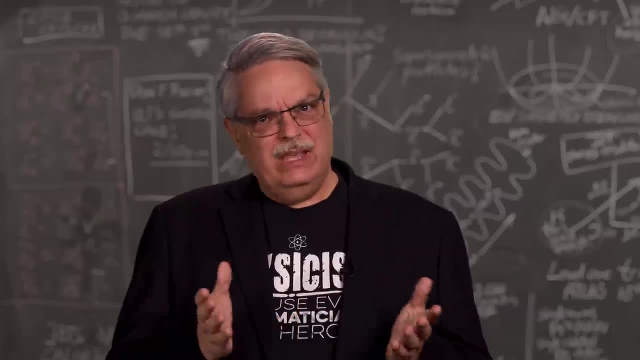 discrete object, what scientists call a particle. So what is a particle? Well, a particle is a particle that is made up of a number of waves. Waves don't seem to be relevant, However, in the world of the super-tiny, the. 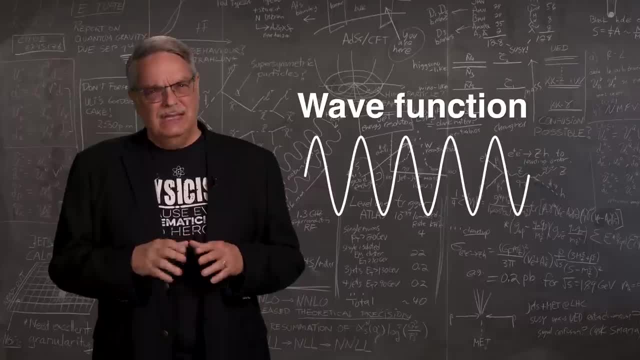 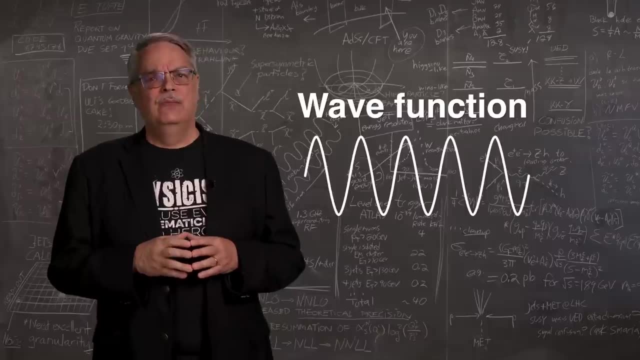 wave function is the only way to explain what's going on. Now. exactly what the wave function actually means is a lot trickier than you'd think. I'll get to that in a little bit. Answering that question is a big part of the reason. 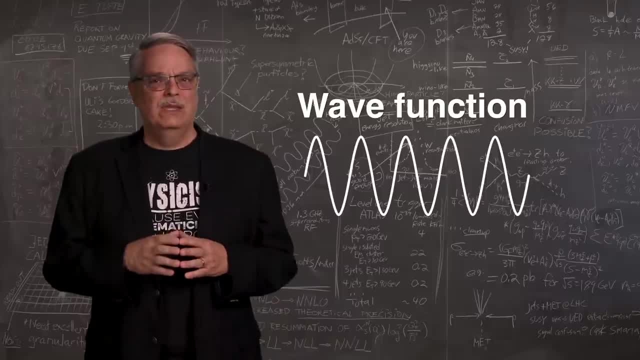 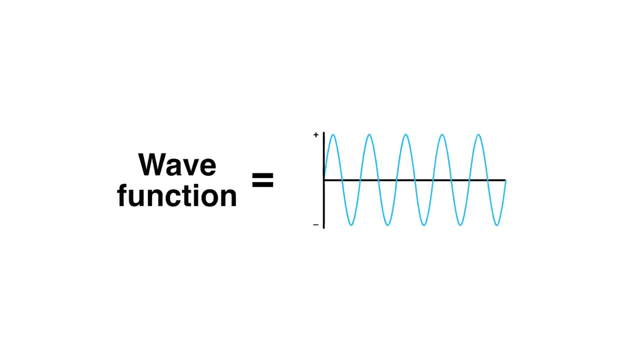 why conversations about quantum mechanics are so mind-blowing. However, there are ways we can think about the wave function that are easier to understand. If we take the wave function and square it, which means to multiply it by itself, the squared wave function tells: 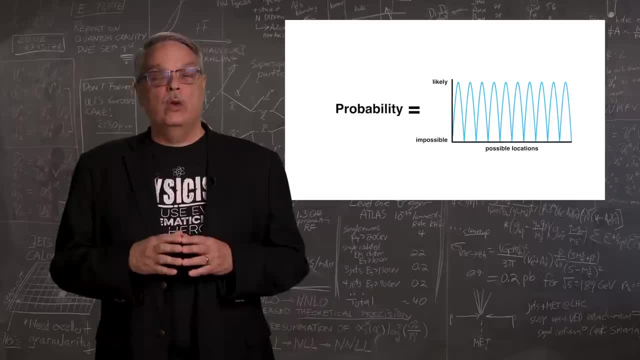 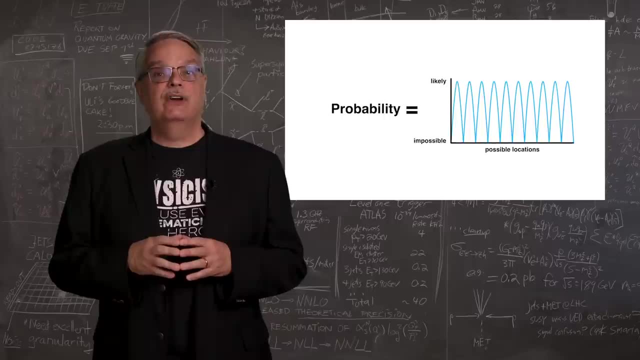 you where a particle can be found. Where the wave function is large, there is a large probability of finding the particle there, and where it's zero, the probability of finding the particle there is zero, So that's not too bad. The wave function squared gives you the probability. 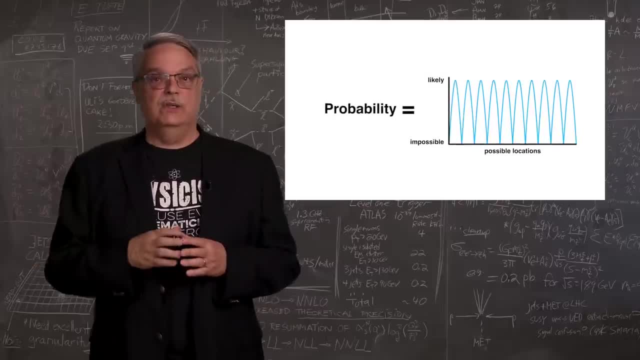 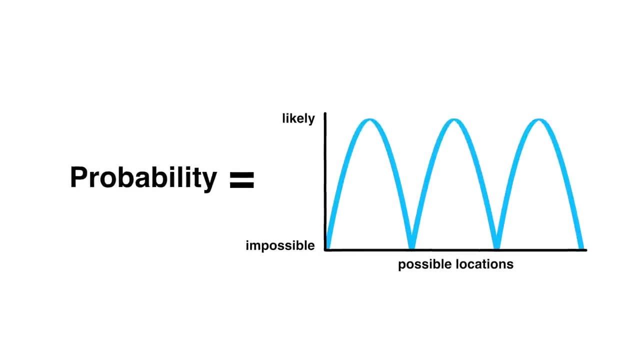 of where you can find the particle. the wave function is describing. That's the first big quantum idea. Now when we detect the particle, say the electron or photon, we don't find it everywhere. We find it in one location At the moment of detection: the location of the particle. 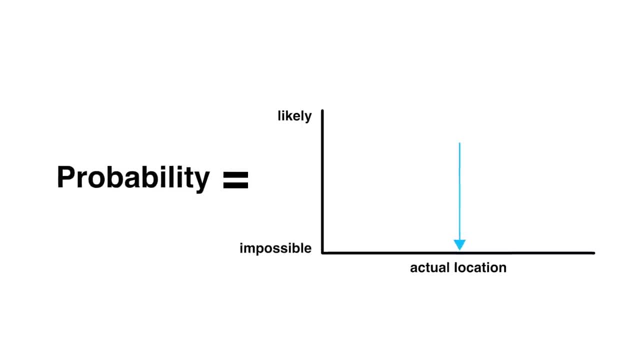 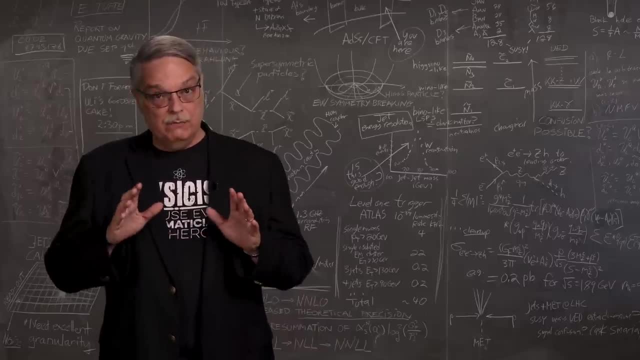 is determined. Scientists call this moment of detection the collapse of the wave function. There's a reason for that particular phrase, and it's because of a quantum weirdness: When you roll a fair die, there is a probability that each side will come up. 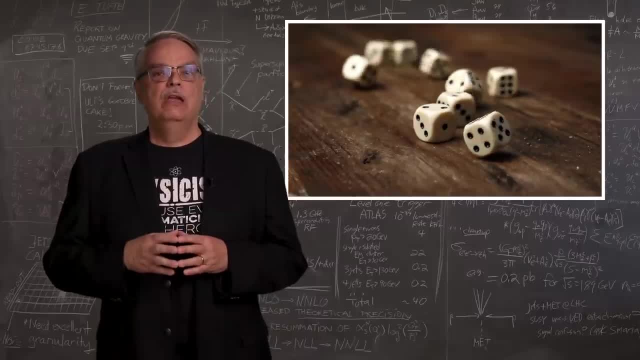 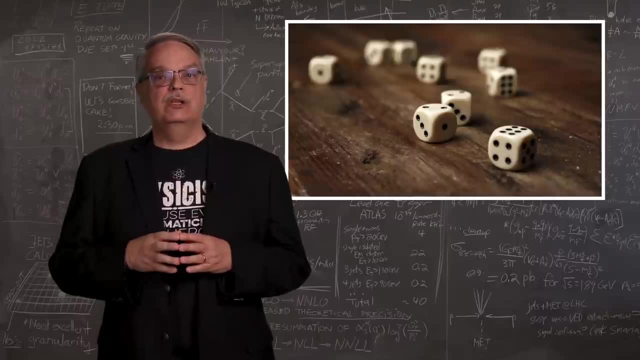 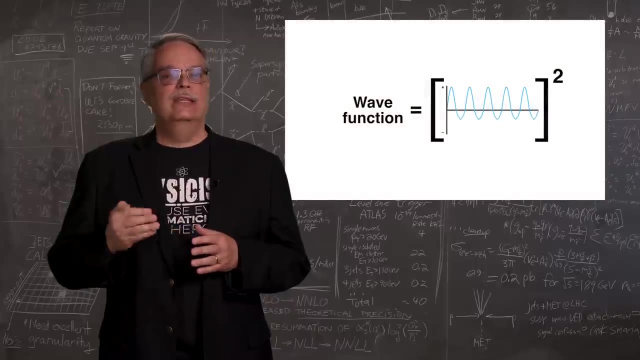 It's difficult to predict which side we'll see when it starts rolling, but if we knew the cube's original velocity and the details of the surface that it's rolling on, we could reliably predict the top face of the die. In quantum mechanics it's different. In quantum mechanics, the electron or photon- 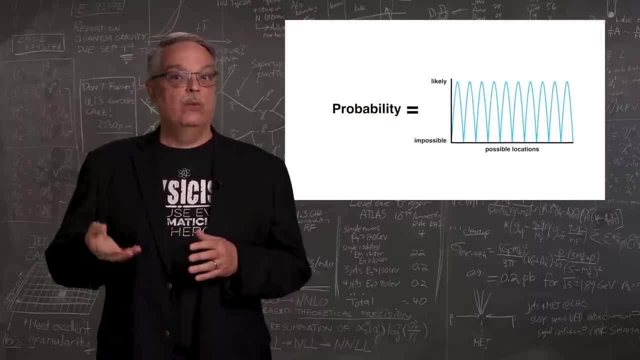 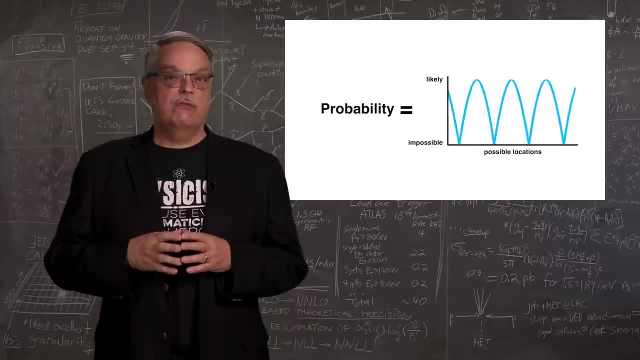 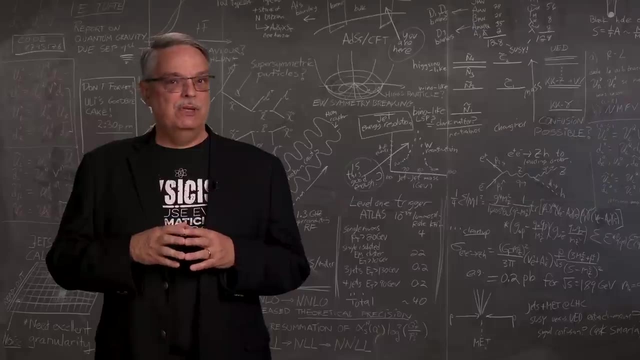 is actually in all locations allowed by the square of the wave function, and it is at the moment at which the particle's location is detected that the wave function changes. in many locations to the one location where the particle is found, The wave function collapsed from being in many locations to just one. 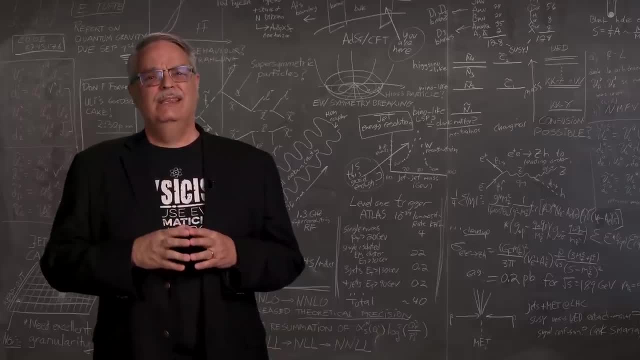 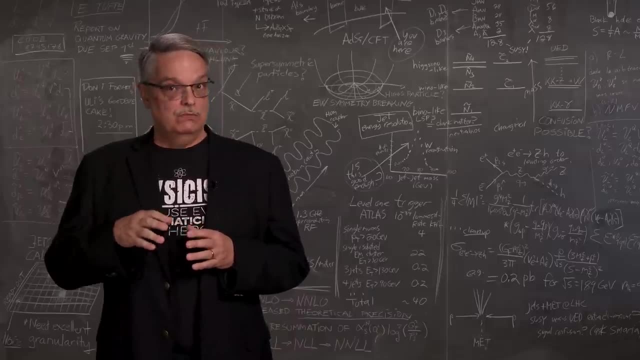 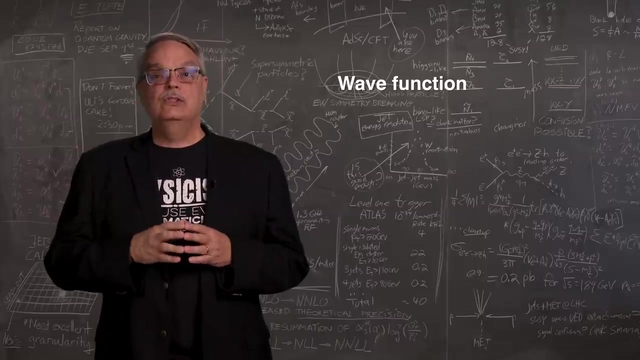 So those are the two key components of quantum mechanics. Now, before we get into just why quantum mechanics still seems so mysterious, it's worth stating the things on which most scientists agree. There is a mathematical function, called a wave function, that, when you square, it tells: 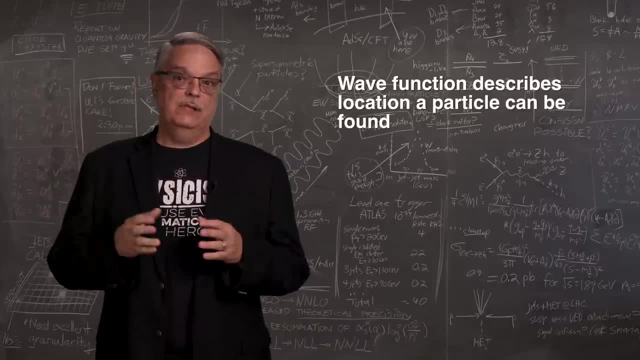 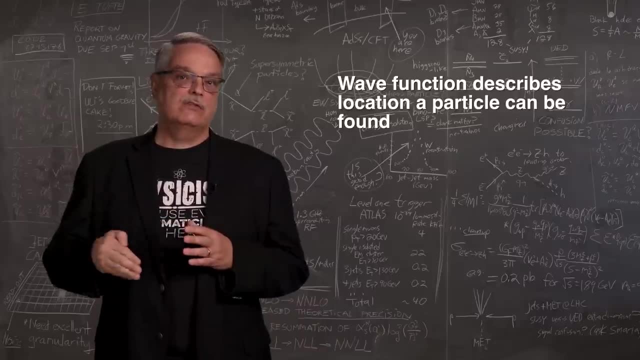 you that you can find the subatomic particle, and with what probability? The subatomic particle is simultaneously everywhere. the wave function says it can be kind of like the electron or photon being spread out, And then, when the particle is detected, the wave 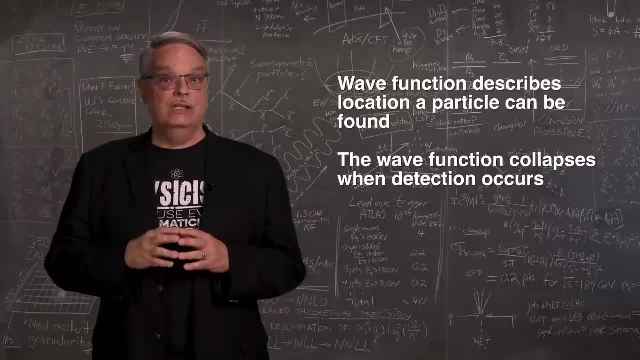 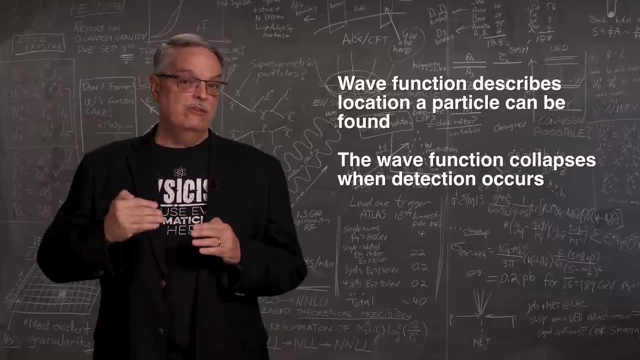 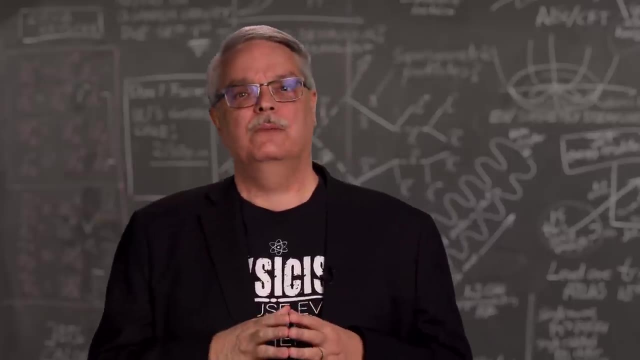 function collapses, and then we know with 100% certainty where the subatomic particle is. There is nearly universal agreement that this way of thinking about things gives accurate predictions. So just what is so confusing about quantum mechanics? Well, it boils down to the very 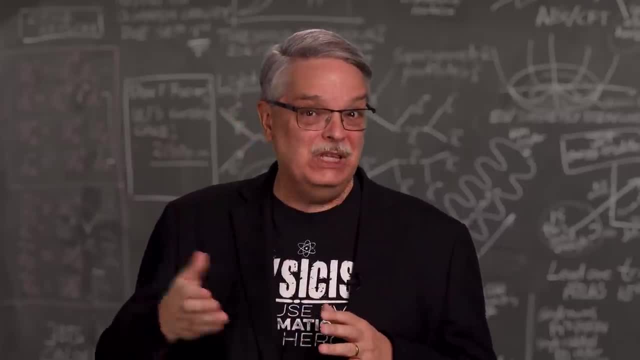 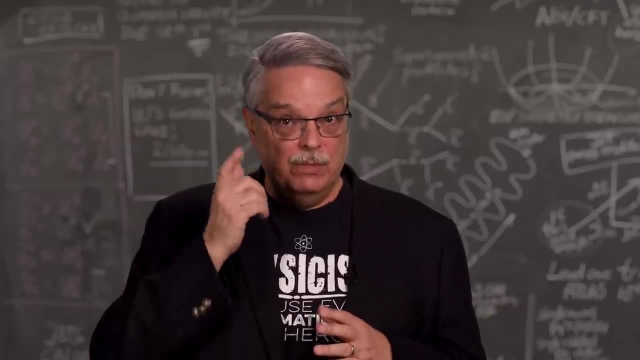 simple fact that nobody really knows what the wave function really is. I mean, we know how to use it to make predictions. That's what's been called the shut-up-and-calculate school of thought. But the true nature of the wave function is perplexing. The simple 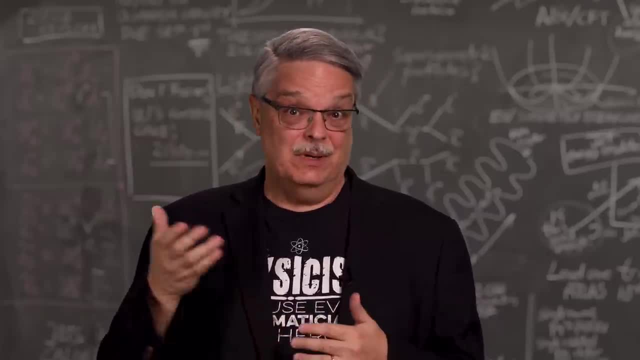 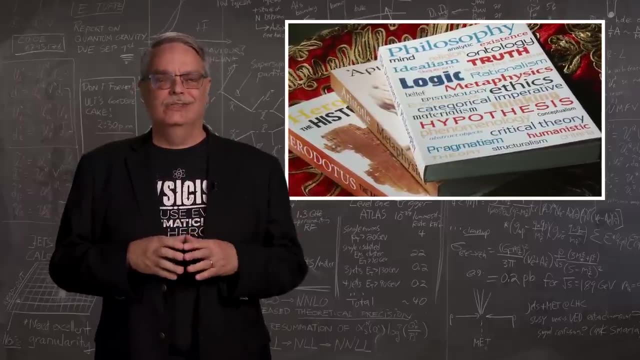 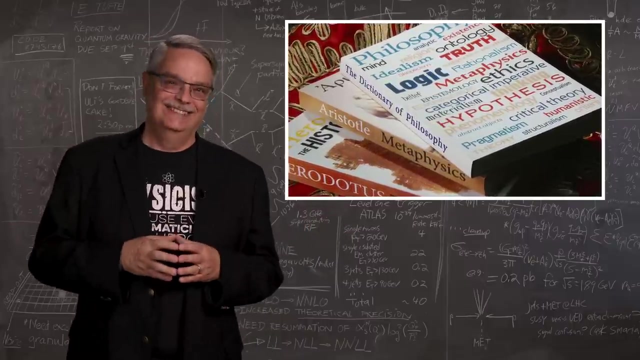 and honest fact is that, despite a century of thinking about it, nobody knows what it is. There are philosophers who argue about whether the wave function is an ontological or epistemological construct, And those are big words because, well, you know philosophers. 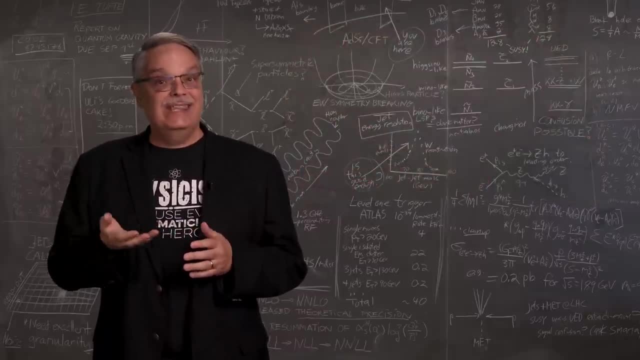 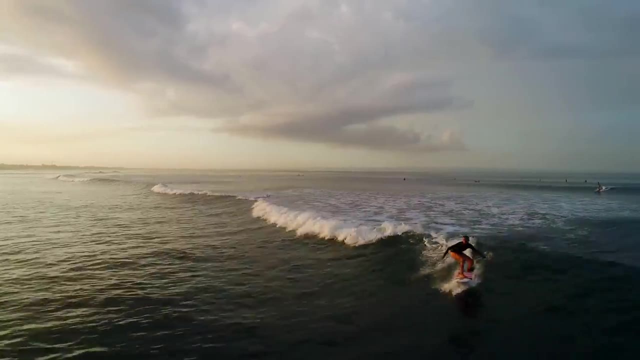 Then there are some people who claim that the waves are actually things that just push other things around. They'd say that the electrons are particles getting pushed by the waves like surfers on a gnarly curl at Oahu, The technical term in quantum mechanics. 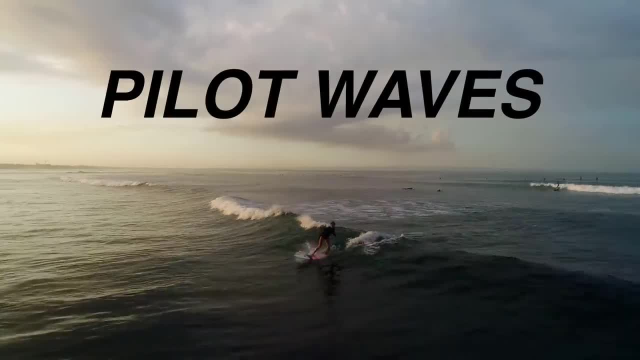 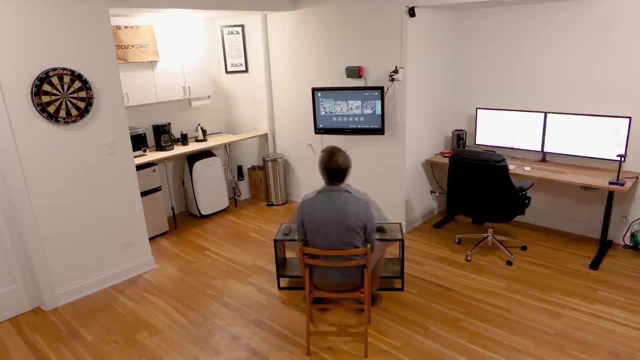 for this idea is pilot waves. Another school of thought says that the wave function predicts what can happen, and when you collapse the wave function, you literally create several universes in which each one one of the possible outcomes occurs. This is called the many worlds interpretation. 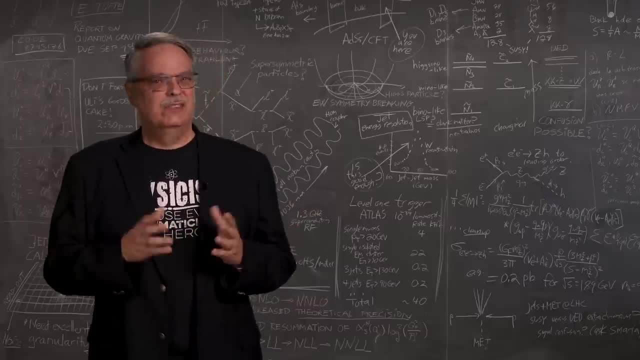 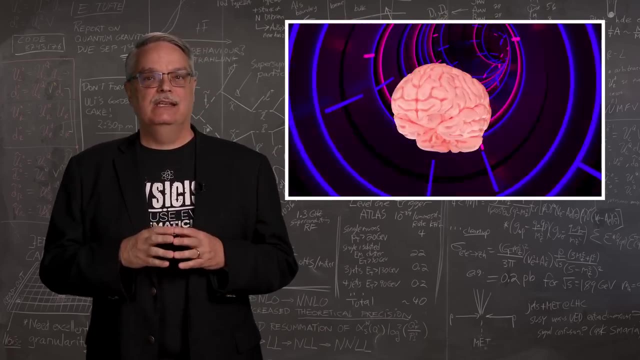 So which one of these ideas is right? Nobody knows. It's truly a head-scratcher. And because science hasn't figured it out yet, that opens up the conversation to weird ideas like the mind-body problem of traditional philosophy or the idea that there's no. 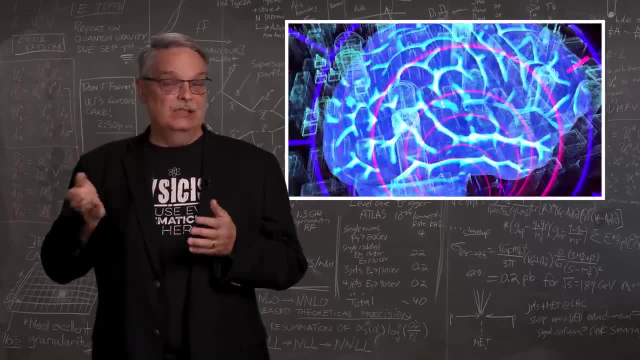 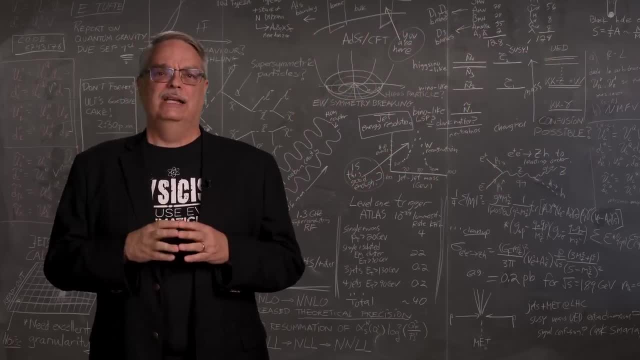 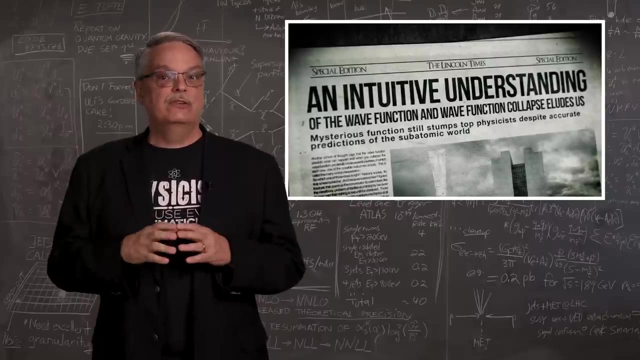 real philosophy, because it's been said that nothing is real until it's observed. Those things really aren't connected to quantum mechanics at all. This is the bottom line. We know how to use the wave function to make accurate predictions of the subatomic world, and yet we don't have a fundamental understanding of the wave. 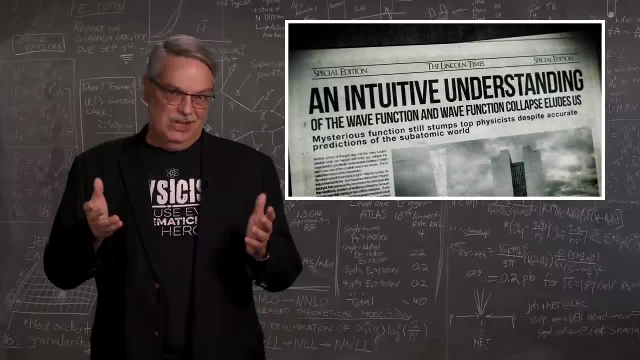 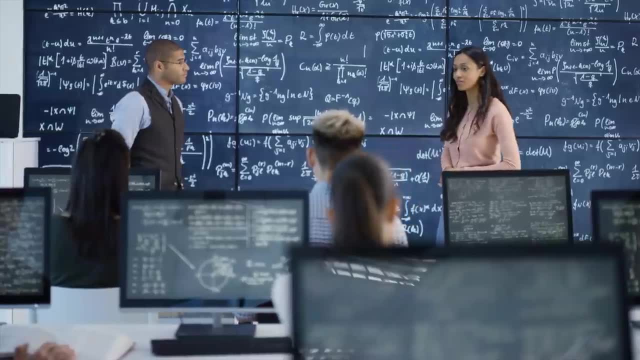 function and what happens when it collapses. This is a not-so-secret secret of physics And it's not for lack of trying. Many people have mulled things over and generally said: I've generated tons of ideas, but none of them have resulted in a definitive conclusion. 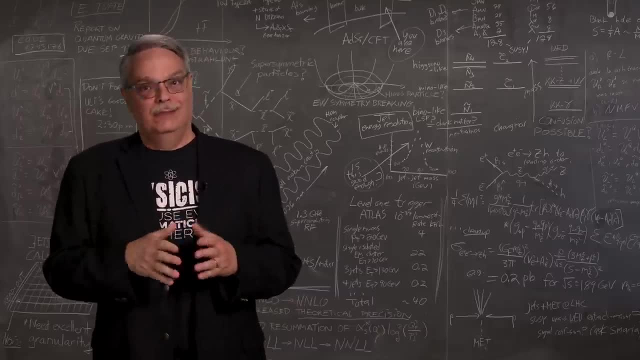 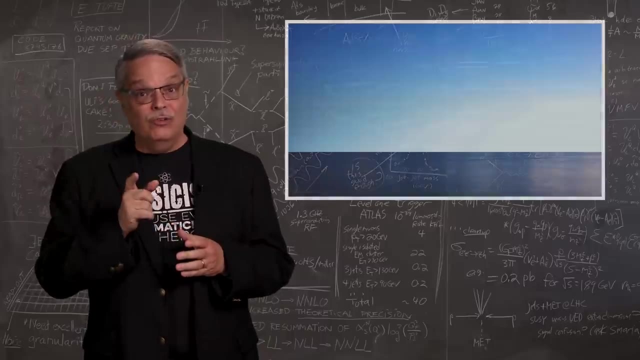 It's a dissatisfying state of affairs, to be sure, but it is what it is, and it's going to take a genius to move us forward. For the time being, we'll just have to wait and see, And hopefully you now know enough to dismiss any explanation that invokes zombie. 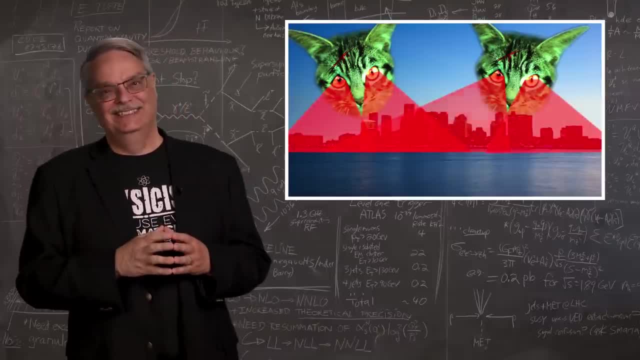 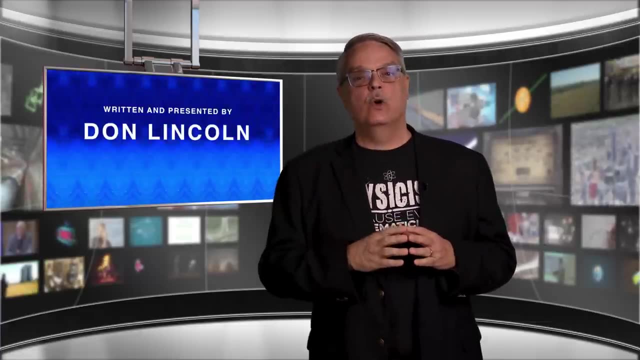 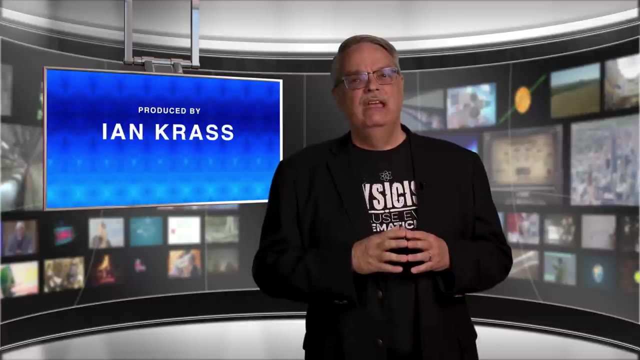 cats that generate reality by looking at it. So I hope that this video was eye-opening and that it kind of gave you a sense of the key ideas of quantum mechanics And hopefully you can see why books written for the public about quantum mechanics can be kind of sketchy.